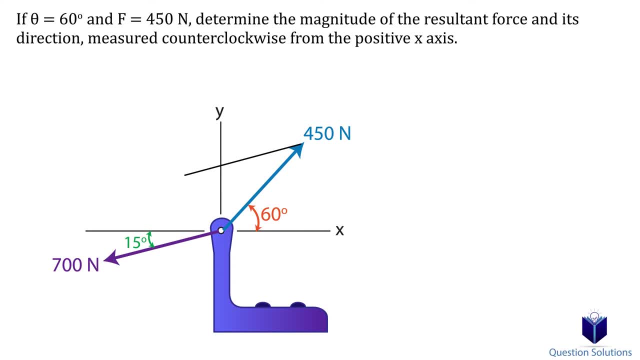 The first step is to draw a line that is parallel to the 700 newton force. Next a line that's parallel to the 450 newton force. Notice how this creates a parallelogram. You can see that the line is parallel to the 750 newton force. Notice how this creates a parallelogram. 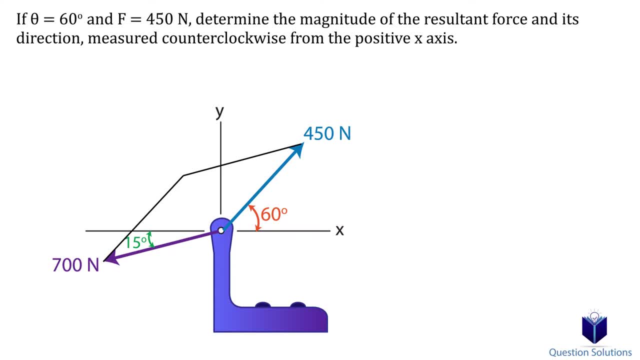 The name for this law comes from. Now, if we draw another arrow, starting from the origin to where these two lines intersect, that's our resultant force vector. It's the diagonal of the parallelogram. Notice also that we have two triangles formed. You can solve this problem using either of the. 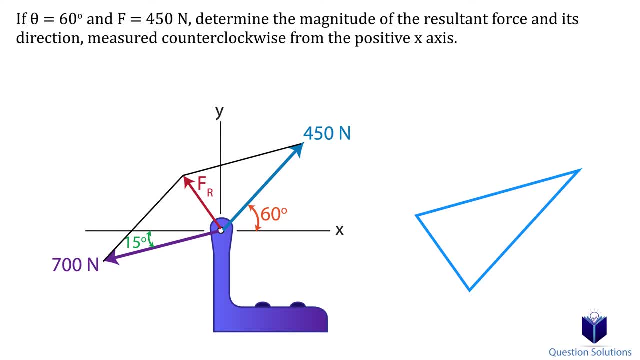 triangles. I'm going to pick the one on top and move it out. So one side of the triangle is 450 newtons and the other side is 700 newtons. To find the remaining side, we can use the law of cosines. 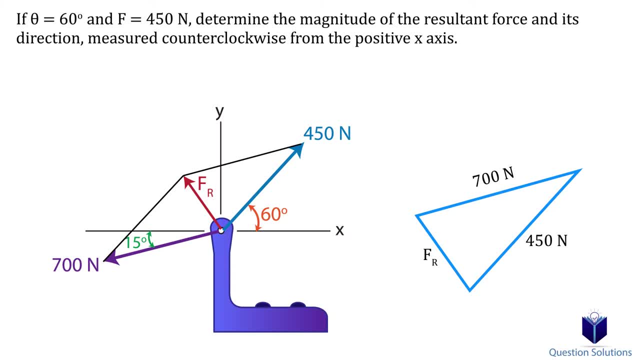 But to use it we actually need an angle inside the triangle. The easiest one to figure out is actually the top angle. If we draw a line parallel to the x-axis at the top, then the whole angle has to be 60 degrees because it's an alternate interior angle. Now we know that the 700 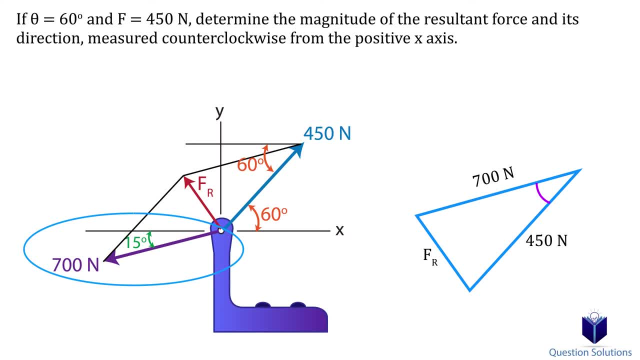 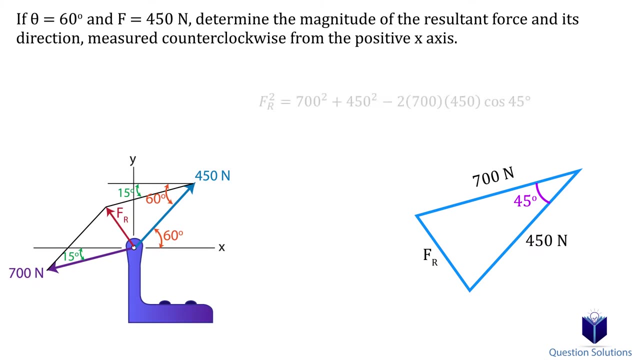 newton force is 15 degrees below the x-axis, which means the angle between the x-axis parallel line and the 700 newton parallel line is 15 degrees, at the top as well. So if we subtract one from the other we get 45 degrees. Now we can apply the law of cosines. Let's solve Just. this value isn't a. 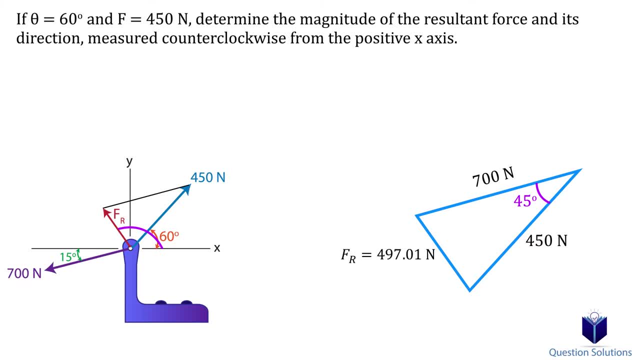 complete answer. We need an angle to show the direction of the resultant force, since it's a vector. So what we need is to find the angle it makes with respect to the x-axis. So first let's find the bottom angle in our triangle. For that we can again use the law of cosines. 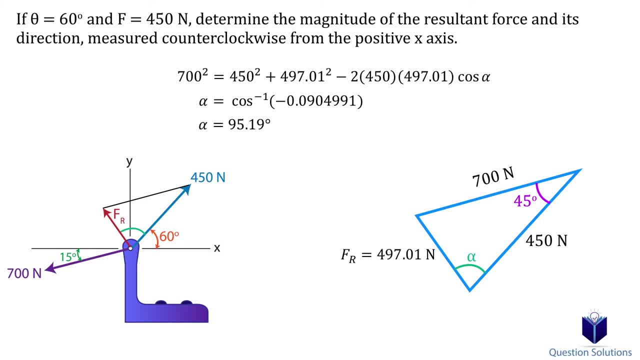 Solving gives us the angle inside the triangle. To get the full angle from the other, we get 45 degrees, the x-axis. all we need to do is add the 60 degrees. So the answer to our question is both of these parts. Let's take a look at this question where we need to figure out. 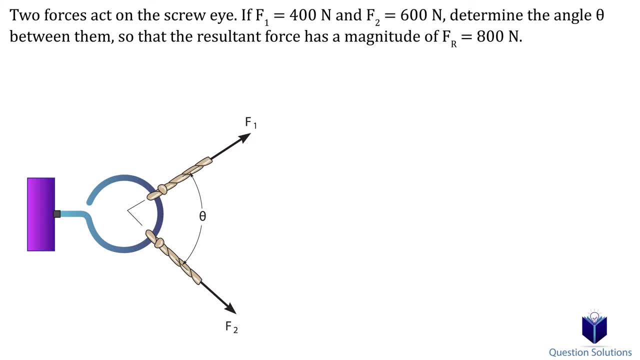 the angle between the two forces, so that the resultant force would have a magnitude of 800 Newtons. So the first step is to draw the parallel lines, starting with the 400 Newton force. Now for the 600 Newton force. Next we draw our resultant force to the point.